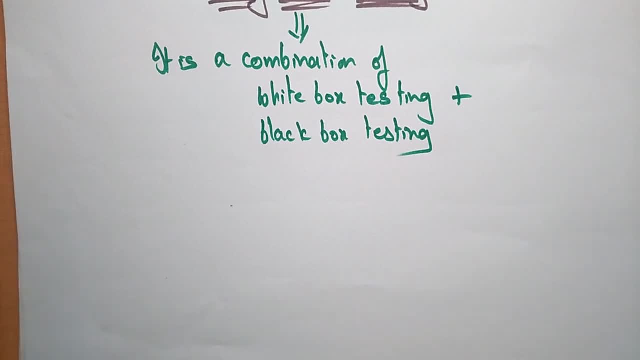 box and black box testing. Now let us see The first thing you have to write. the first thing you have to write is that whenever they ask about what is a grey box testing, it's just a combination of white box testing and black box testing. So it is a strategy for the software. 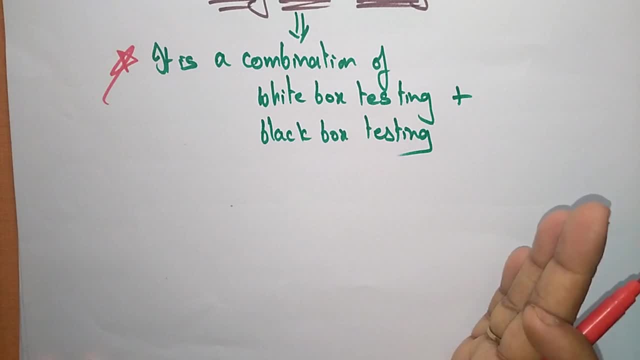 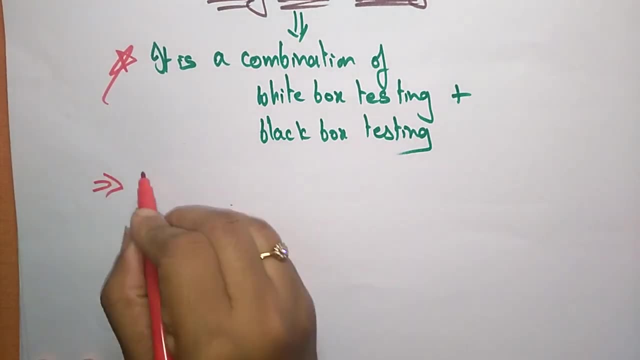 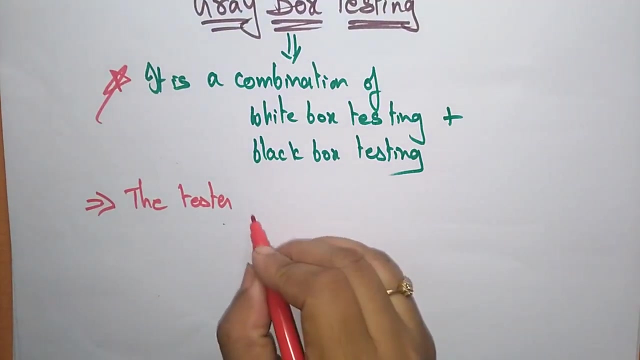 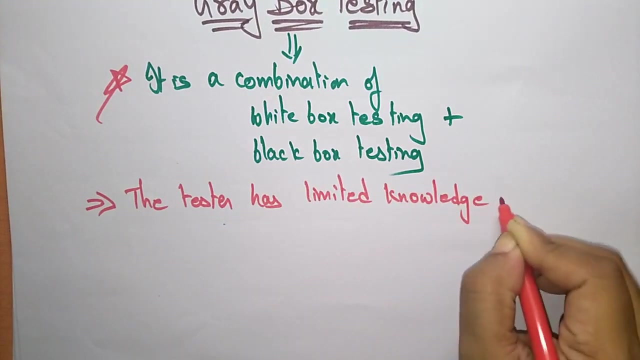 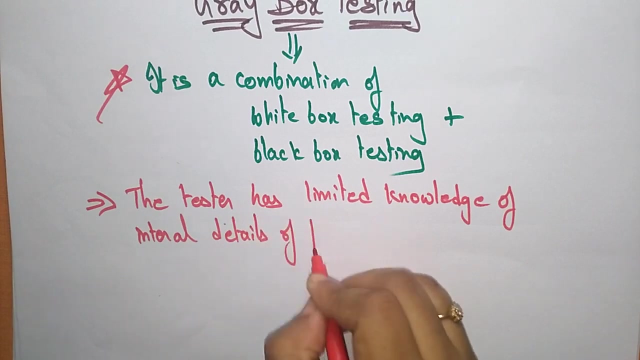 debugging in which testers has limited knowledge of internal details of program. So they are having the only the limited knowledge the testers have who are going to test the grey box test by using grey box testing. Those testers has limited knowledge. There are limited knowledge of internal details of a program. The person who is using a tester. 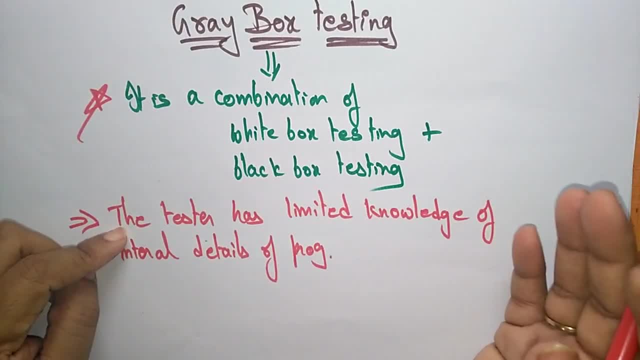 is using the grey box testing, he is having the limited knowledge of internal details. So if he is having limited knowledge then he can go for the grey box. So it completely depends upon the tester who is having limited knowledge. So essentially you can say that loose and 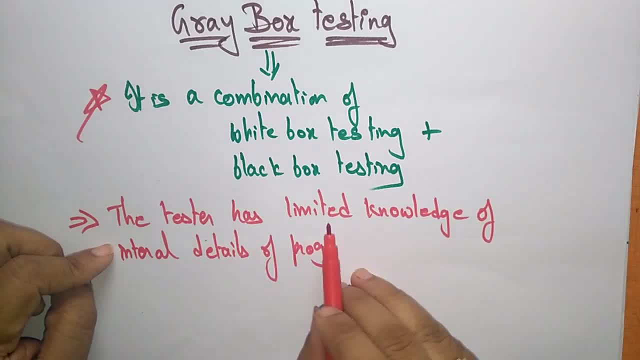 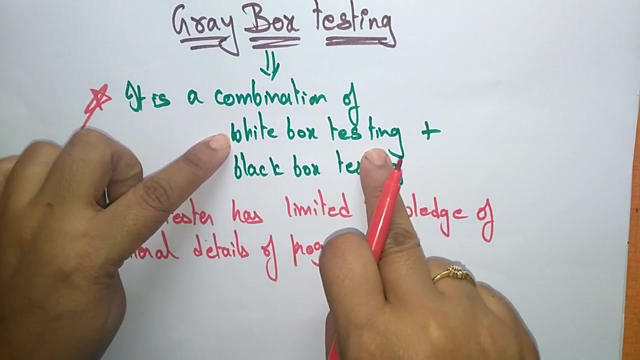 tester who is going to test on the project. so if it is having a limited knowledge, then it is preferred gray box. so means what is the black box testing? there is no knowledge of internal coding, okay. and whereas white box testing is completely depends upon internal structure, internal details, 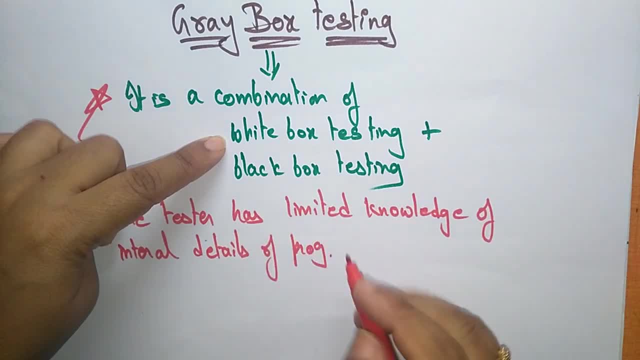 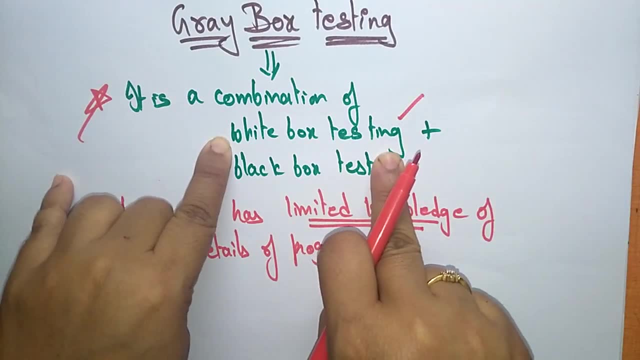 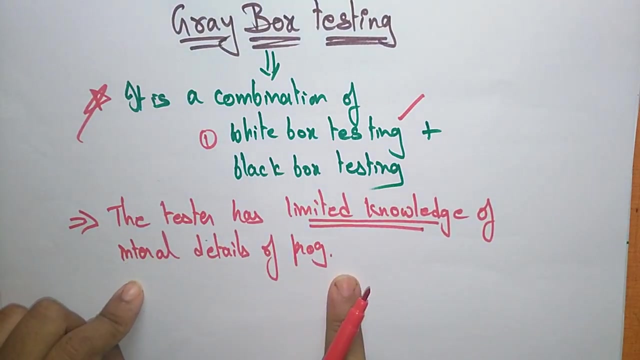 of a program. so here i am saying the tester is having the limited knowledge. so if it is, if he is having the limited knowledge means okay, it is a combination of white box testing. so the first case will be true: the tester has limited knowledge of internal details of program. if it is, if he is, 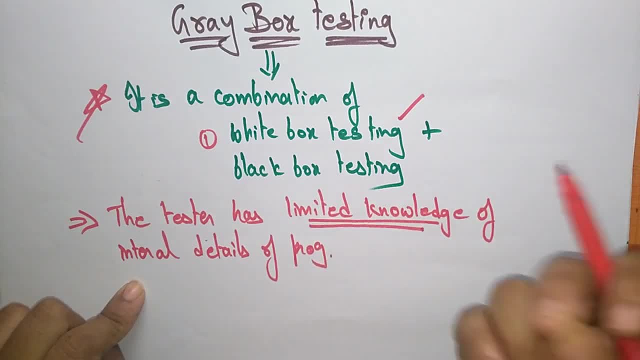 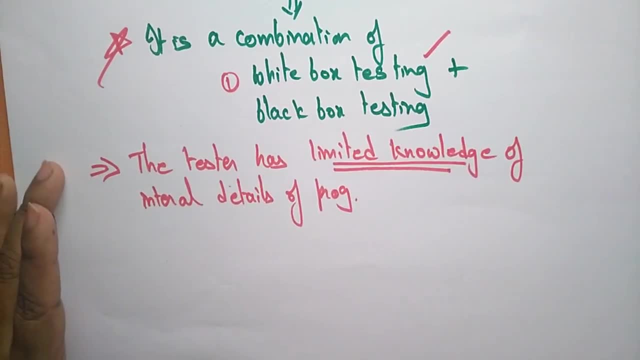 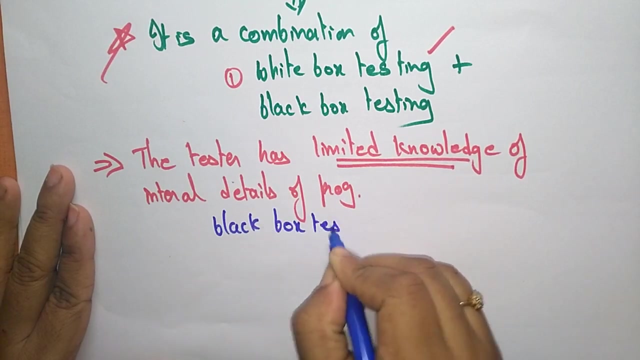 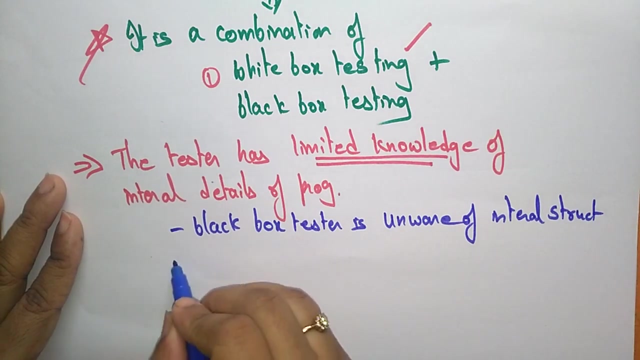 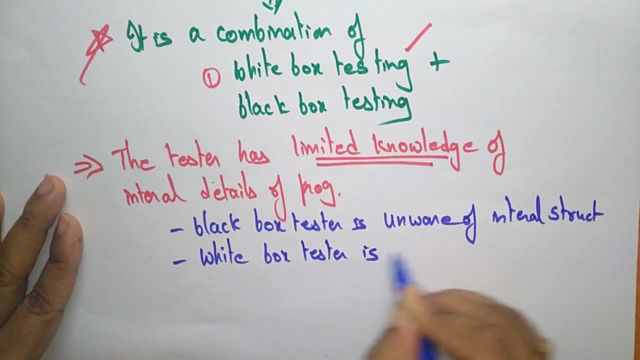 having the limited knowledge or complete knowledge. then it is white box testing. next, the black box tester is. let me write that the black box tester is unaware of internal structure, unaware of internal structure of system and whereas white box testing, the white box tester is aware of, aware of internal structure of system. 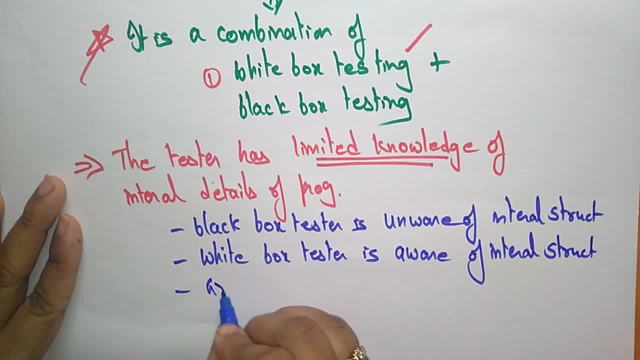 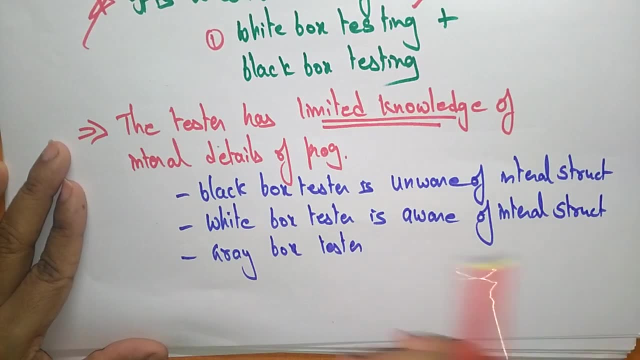 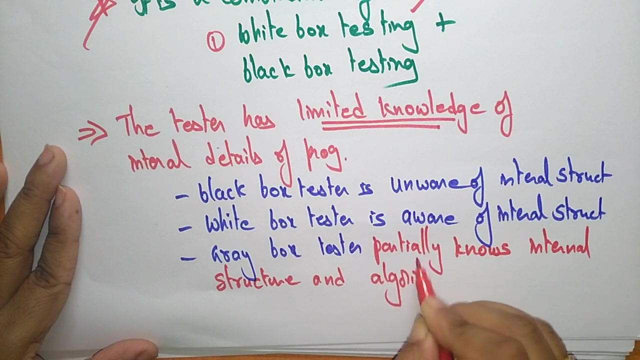 whereas Gray box testing, gray box tester is. let me write that a gray box tester partially, partially, knows internal structure, and here I am saying, and So he is partially knows the internal structure. that is, a white box testing. and algorithms, algorithms of defining test case, defining test case. 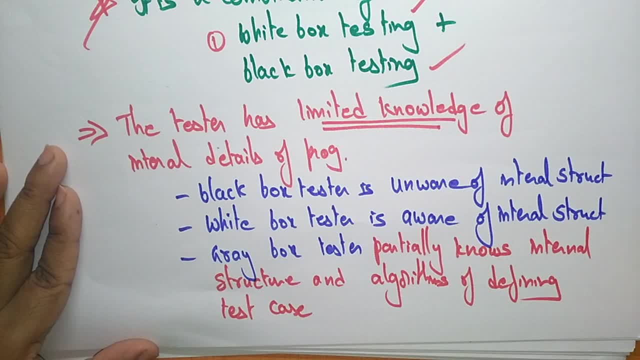 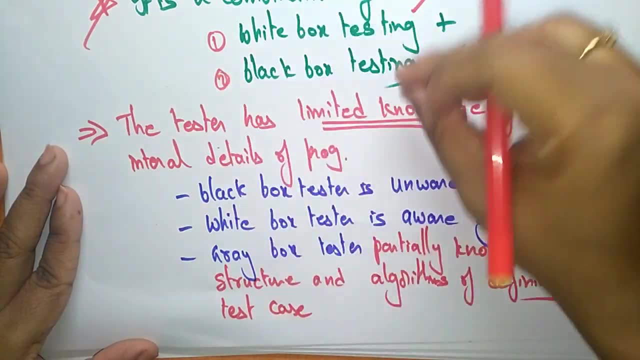 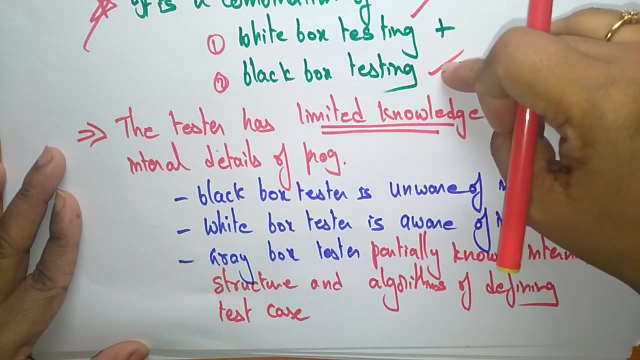 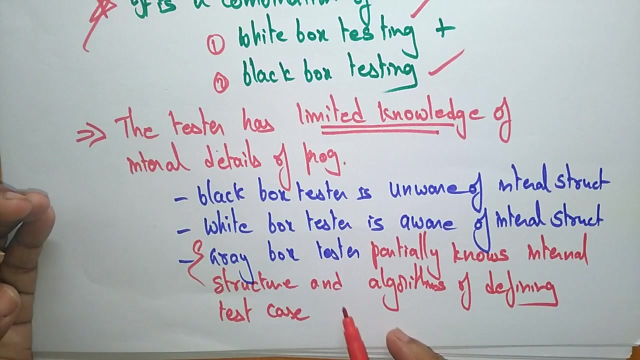 That means it is the functionality of the structure. functionality of the system is also knowing. So that means black box testing. So it is satisfying both. the condition It that gray box testing is having the limited knowledge You offer, internal details, and it is having the idea about the algorithms of definition of the all the test cases. So that's why the gray box testing is a combination of both the white box testing and black box testing. 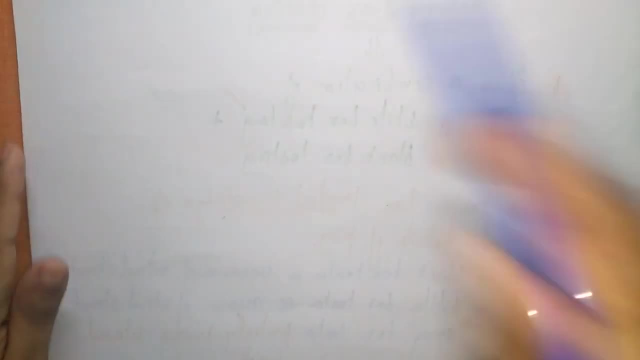 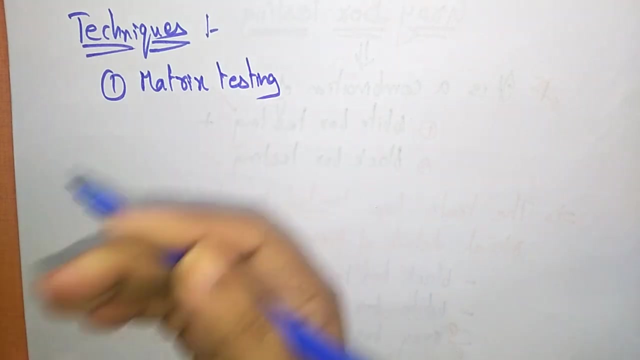 Now let us see the techniques of gray box test. I hope you understand what exactly the black box, white box and the gray box techniques. First technique is matrix testing. So here the matrix testing states the status of report of the project. Just, it states the report of the project. 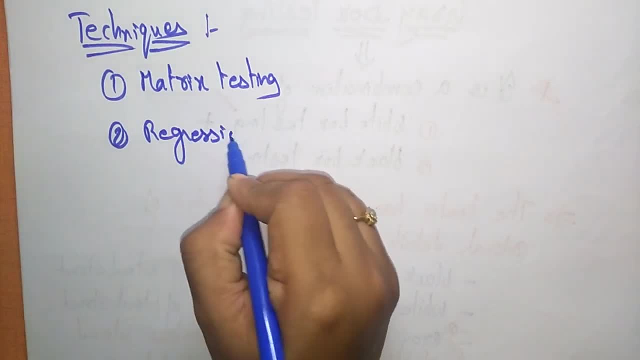 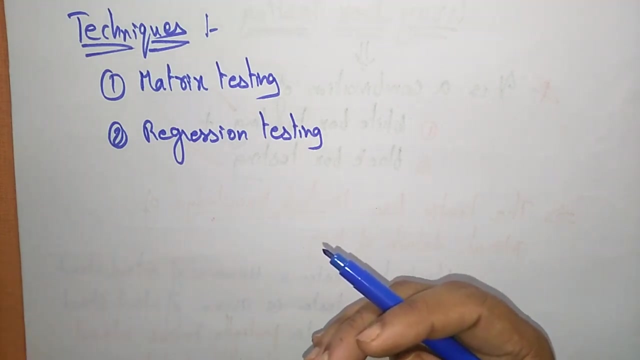 Next is a regression testing. Regression testing here just rerunning of the test cases If any new changes are made, just it is always. rerunning the test cases means if still any errors again, it's checking again errors will come in. It's just rerunning of the test cases. 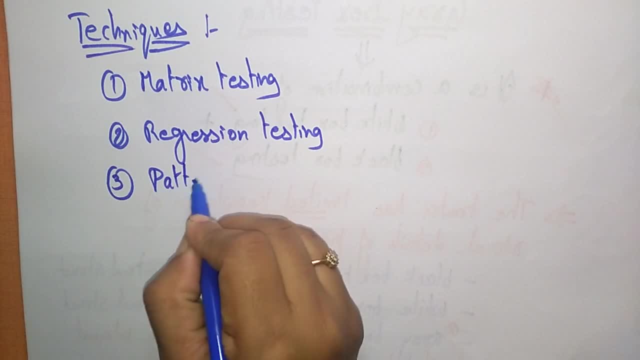 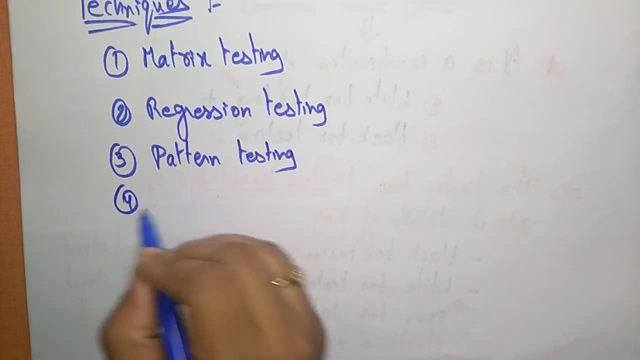 Third: pattern testing. So the pattern testing is also rerunning of test cases If any new changes are made. Fourth one is orthogonal array testing. So what is this orthogonal array testing? Here this orthogonal array testing is used as a subset of all possible combination. 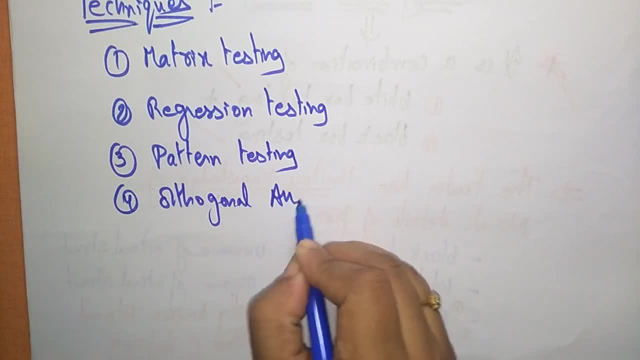 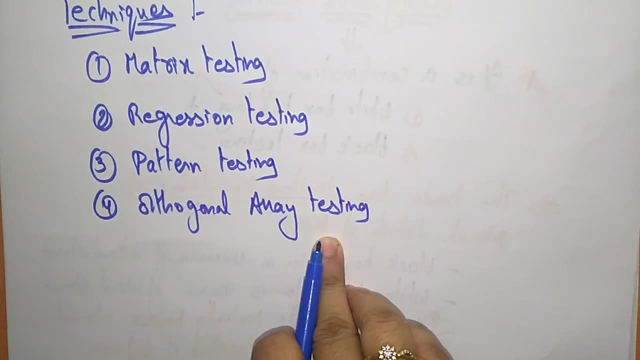 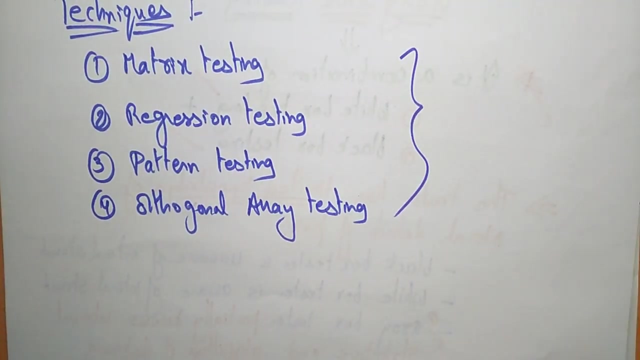